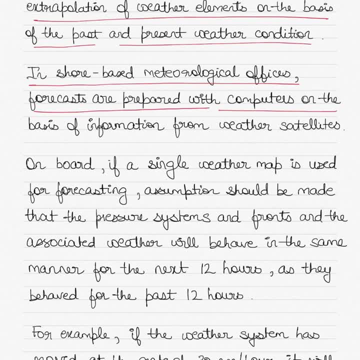 forecasters are prepared with computers. They have sophisticated computers on the basis of information from weather satellites. So they of course have much more data, much more equipment, better analysis capability and they provide you detailed analysis, But on board of. 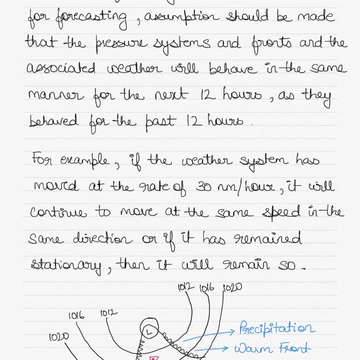 course you are not. you do not have access to such sophisticated computers, So that's where your skills come in. All right, so on board. of course, if a single weather map is used for forecasting, assumption should be made that the pressure systems and fronts and the associated weather, 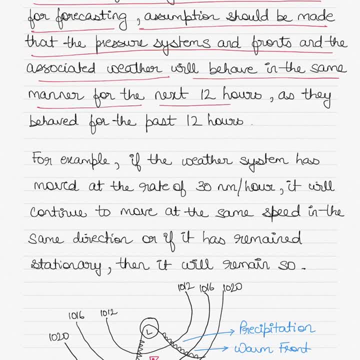 will behave in the same manner for the next 12 hours as they are behaving for the past 12 hours. So, like I said before, this is all based on the assumption that, however the weather has behaved in the past, this is how the weather will behave. 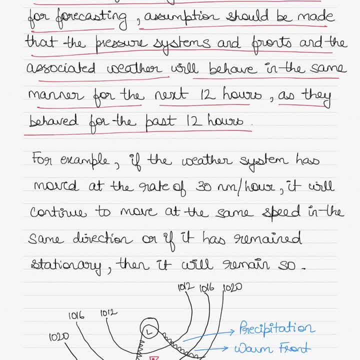 in the next 12 hours, although there could be slight changes which you cannot predict. It's only can be predicted, maybe, by the people sitting in the shore offices, but sometimes even they go wrong, But that happens very rarely, but sometimes because weather can't be predicted so accurately. 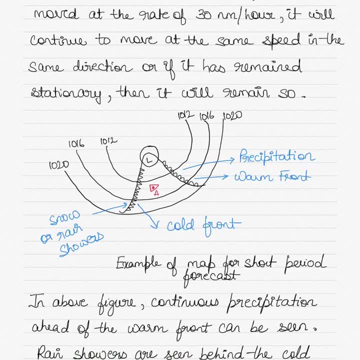 right. So here I've shown you a quick diagram on. I've focused on a particular area of a weather map, especially where the isobars are located. So I've shown you a particular area of a weather map. you know that on your weather map you have isobars drawn everywhere, But here what you will do is: 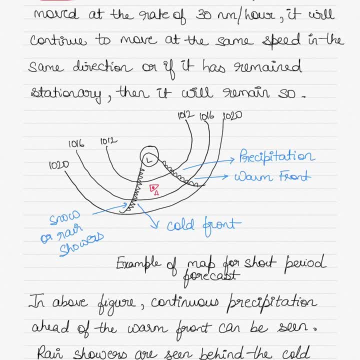 let's see here for the example. for example, if the weather system has moved at a rate of 30 nautical miles per hour, we assume that it will continue to move at the same speed in the same direction. or if it has remained stationary, then it will continue to remain so. So these are the kind of 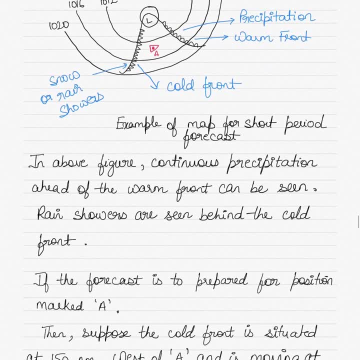 assumptions that we make. We base it on the past 12 hours. Now what I'm showing you in the diagram here is that on the weather map, if we have isobars drawn, then plot your ship's position. your ship's position is plotted as position number A, So this is your ship's position, All right. 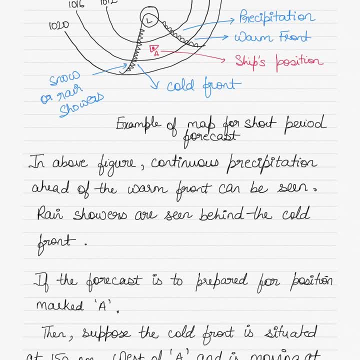 the rest of it. I have drawn it and labeled it already So you can see the isobars are drawn at intervals of four millibars, of 1012 millibars, 1016, 102 Zol. As it is drawn on a weather map. 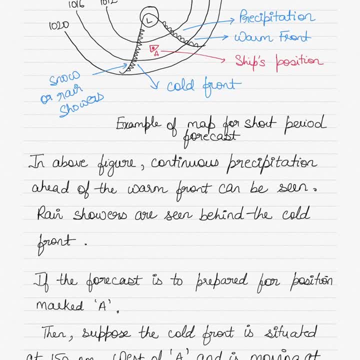 we have the cold front, which are indicated by triangles, and the warm front, which are indicated by semicircles. So you plot the ship's position on the weather map. And then let's take this example of a map for short period forecast. All right, So in the above figure you can see that continuous 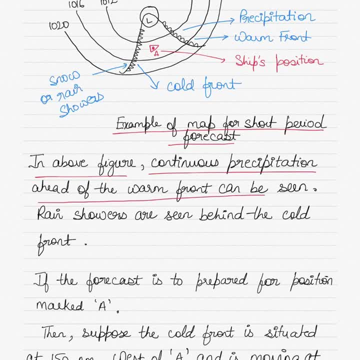 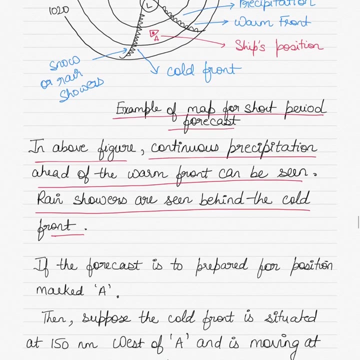 precipitation will be expected ahead of the warm front And rain showers are seen behind the cold front. So you have to figure out your speed and the speed at which this front is moving, And you will know that what kind of weather should you be expecting if you go ahead. 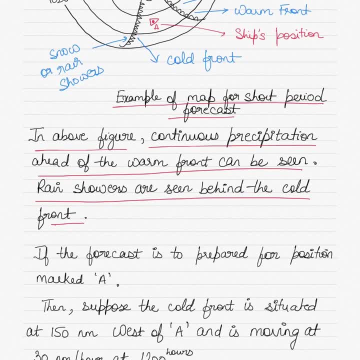 of the warm front or you, the cold front crosses you Alright. So if the forecast is to be prepared for position marked A- that is your ship's position- then suppose the cold front is situated at 150 nautical miles west of position A and is moving at 30 nautical miles per hour at 1200. 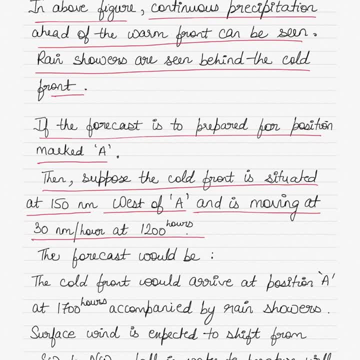 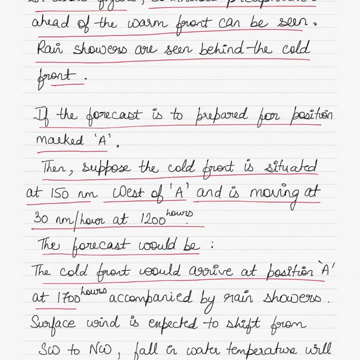 hours. Let's assume that always that will make it easier for us to understand. So the forecast in this case would be that the cold front would arrive at position a at 1700 hours, that's after five hours, because it's moving at 30 nautical miles. 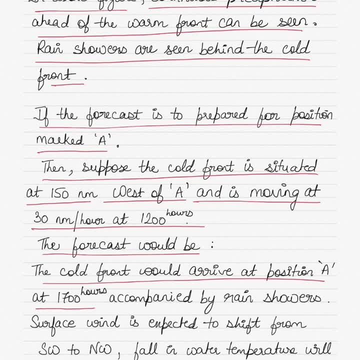 per hour. so 5 times 30 is 150 nautical miles, and it will be accompanied by rain showers, of course. you also have to remember that the ship is moving as well, so it will not be exactly five hours, because the ship's movement depends on the relative speed between the ship and the movement of the 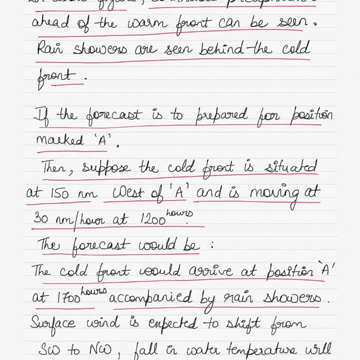 front. but here we are just taking it as a simple case. let's say the ship speed is very slow and the front is moving at that speed, all right. so surface wind is will be expected to shift from the southwest direction to the northwest direction and a fall in the water temperature will also be. 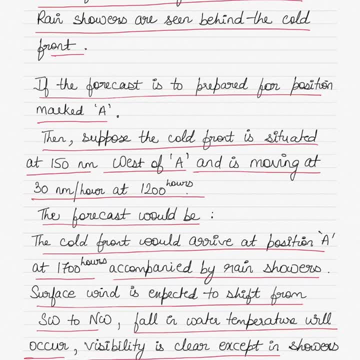 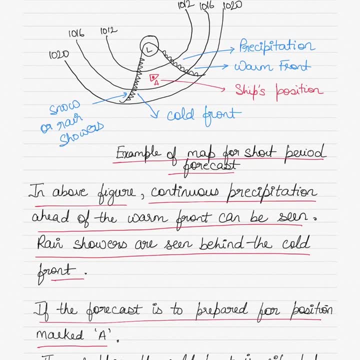 expected to occur and visibility will mainly be clear, except in showers. so remember when a cold front will pass over the ship. the showers, although may be very short in duration, but they are really intense and they are heavy, and visibility is of course obscured because of the intensity of the rain showers, whereas in warm front the precipitation is much less. it's